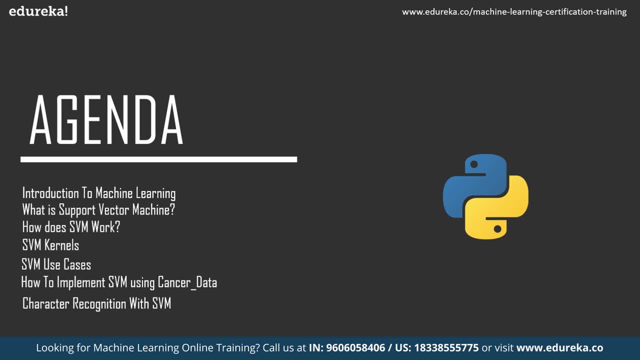 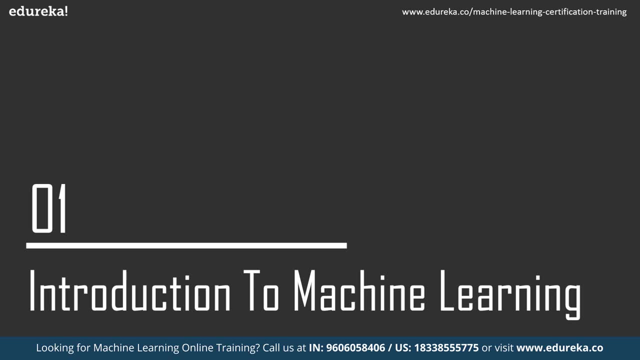 Also do check out the python certification program on edureka. link is given in the description box below. now, without any further ado, Let's try to understand what is support vector machine. But before that let me give you a brief introduction to machine learning. machine learning is the process of feeding a machine enough data. 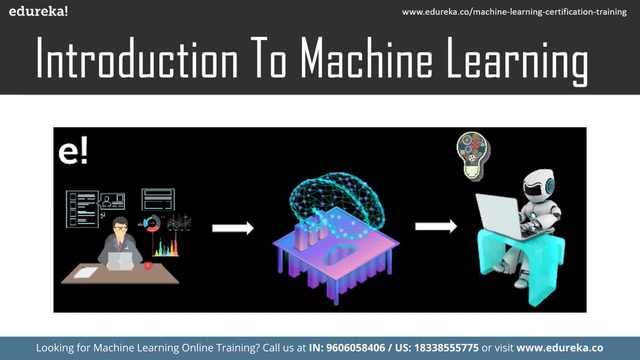 to train and predict a possible outcome using the algorithms at Bay. the more the data is fed to the machine, the more efficient the machine will become. So let us try to understand this with a real-life example. So I'm sure most of you are aware of the predictions made. 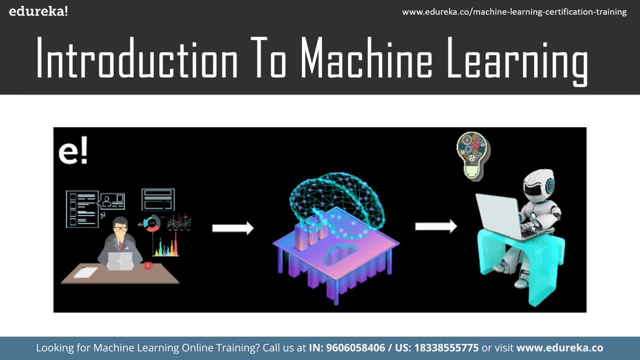 in any sport before any major match. So in this case I'm going to tell you about a football penalty session. Let's say the data of previous performances are considered. So let's say the goalkeeper has saved all the penalties to his right in the last 50 penalties that he has saved. 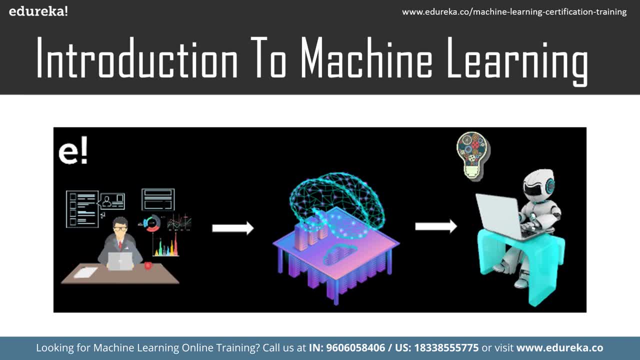 So this data will be crucial to predicting if he will or will not save the next penalty that he faces. Of course, there are other factors to consider as well. Another example is the suggestions that we get while surfing the internet. the data of our previous choices are processed. 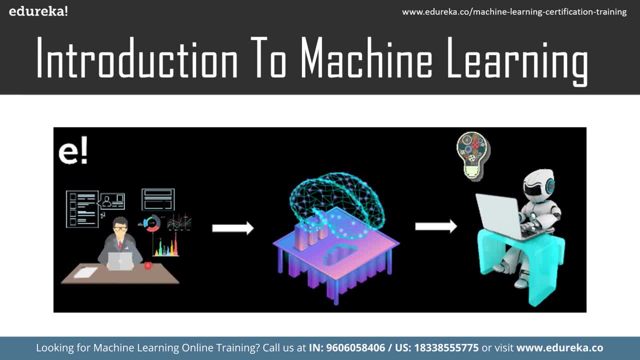 to give us the most favorable content We are most likely to watch. anyhow, machine learning is not just feeding the machine an ample amount of data. There goes a lot of processes, algorithms and decisive factors to get the optimum results. So in this session we will go through one such support vector: machine algorithm. 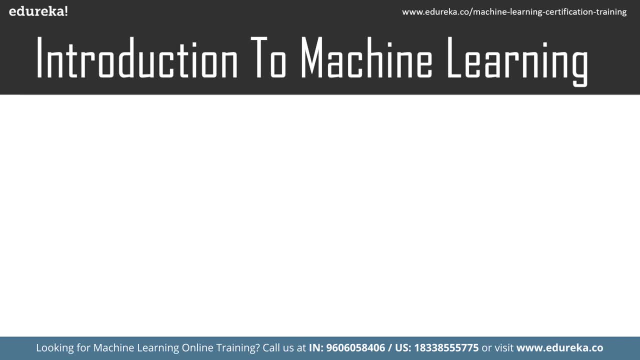 to understand how it works with Python. before that, Let us also take a look at the types of machine learning. So there are three types of machine learning. that is, supervised learning, unsupervised learning and reinforcement learning. supervised learning is contained in a controlled way to oversee the outcome accordingly. 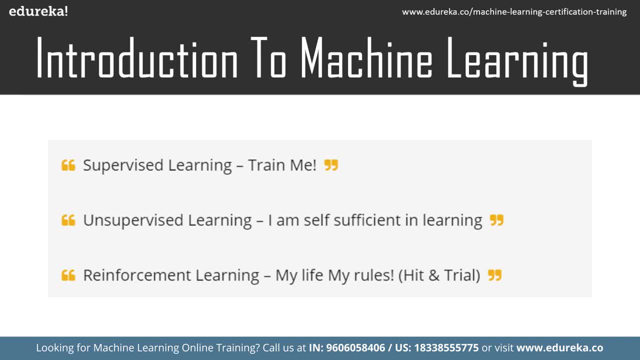 It is, as the name suggests, supervised in a way that the machine learns what the user wants it to learn. coming to unsupervised learning, The machine simply explores the data given to it. The data is sometimes unlabeled and uncategorized, and the machine makes the possible references. 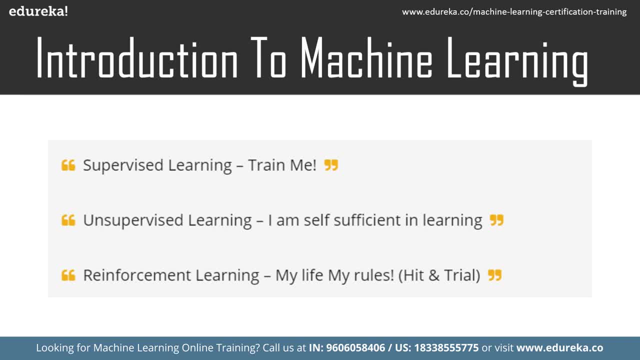 and predictions without any supervision. and talking about reinforcement learning, It basically means to enforce a pattern of behavior. The machine needs to establish a systematic pattern of approach and reinforcement learning. So these are the types of machine learning that we have. Let's move on to the next topic. 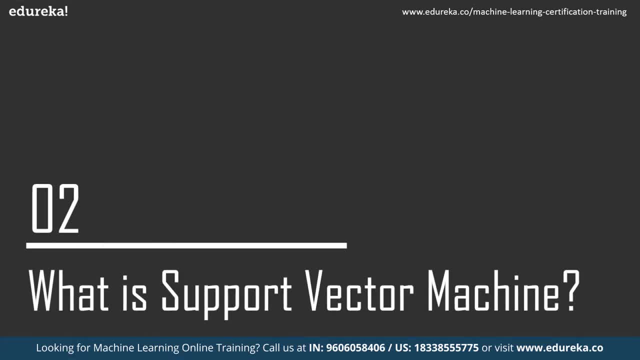 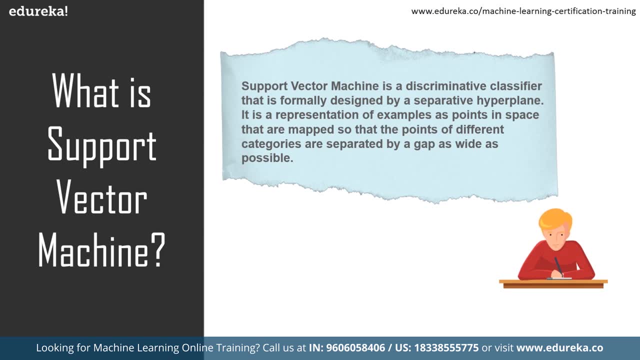 That is, what is the support vector machine. So what exactly is the support vector machine? A support vector machine, or we can call it as SVM, was first introduced in the 1960s and later improvised in the 1990s, and SVM is a supervised learning. 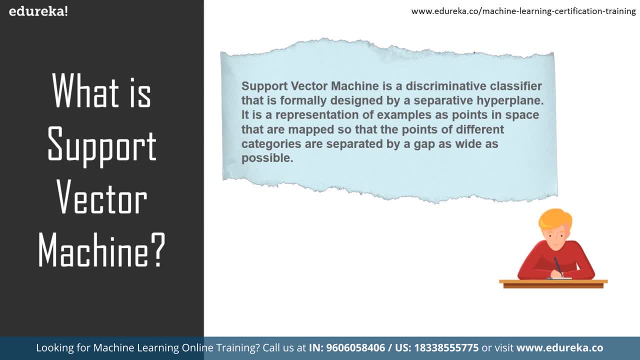 machine learning classification algorithm that has become extremely popular nowadays owing to its extremely efficient results. So an SVM is implemented in a slightly different way than other machine learning algorithms. It is capable of performing classification, regression and outlier detection as well. a support vector machine is a discriminative classifier. 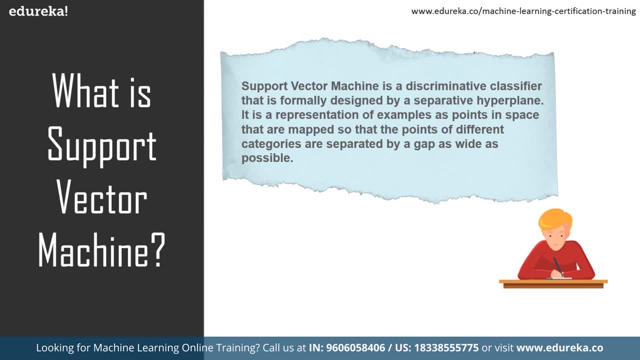 that is formally designed by a separative hyperplane. It is a representation of examples as points in space that are mapped so that the points of different categories are separated by a gap as wide as possible. in addition to this, and SVM can also perform nonlinear classification. 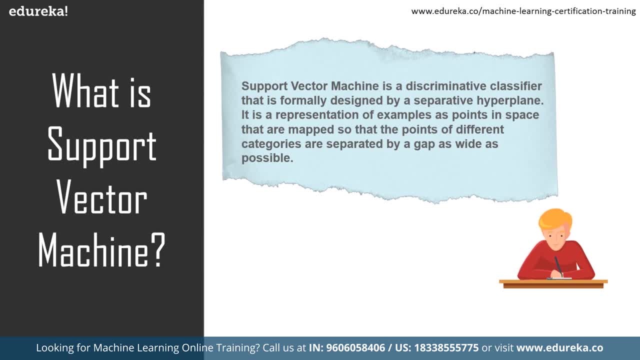 So I'm going to tell you a few advantages and disadvantages of SVM or support vector machine. So, talking about the advantages of SVM, it is effective in high dimensional spaces and it is still effective in cases where the number of dimensions is greater than the number of samples. one more advantages: 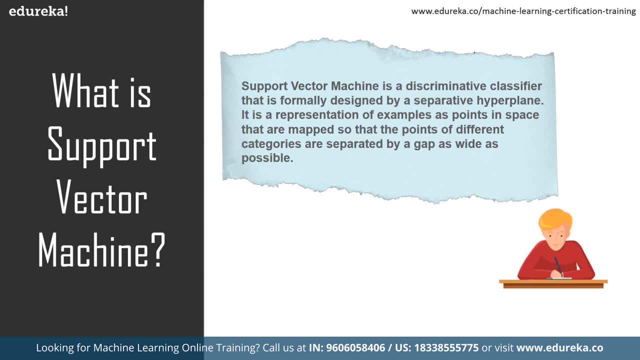 It uses a subset of training points in the decision function. that makes it memory efficient. and last advantages: different kernel functions can be specified for the decision function, which also makes it versatile. coming on to the disadvantages, if the number of the features is much larger than the number of samples we have. 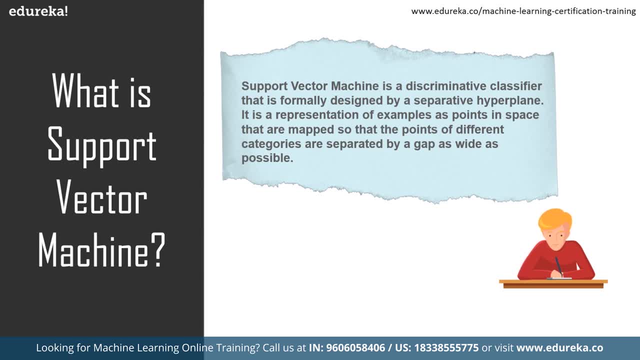 to avoid overfitting in choosing the kernel functions, and regularization term is actually crucial. the next disadvantage is SVMs do not directly provide probability estimates. These are calculated using five-fold cross-validation. So these are the advantages and disadvantages of SVM. Now let's take a look at the next topic. 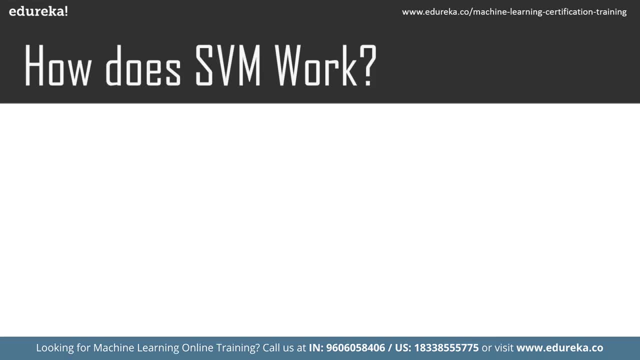 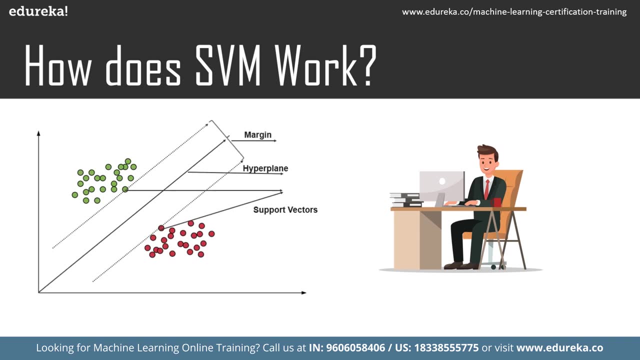 which is: how does an SVM work? So the main objective of our support vector machine is to segregate the given data in the best possible way. So when the segregation is done- the distance between the nearest points is known as the margin- The approach is to select a hyperplane. 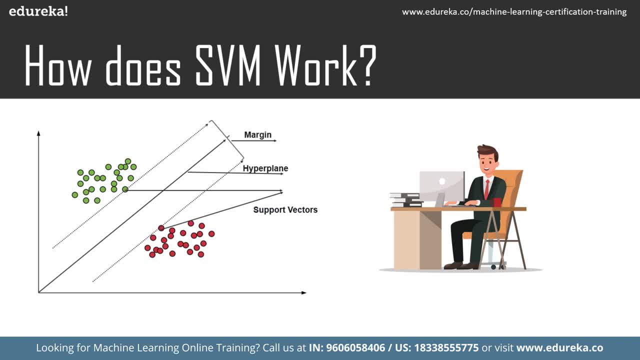 with the maximum possible margin between the support vectors in the given data set. now to select the maximum hyperplane in the given sets, the support vector machine follows the following: it generates a hyperplane which segregates the classes in the best possible way, and then it selects the right hyperplane. 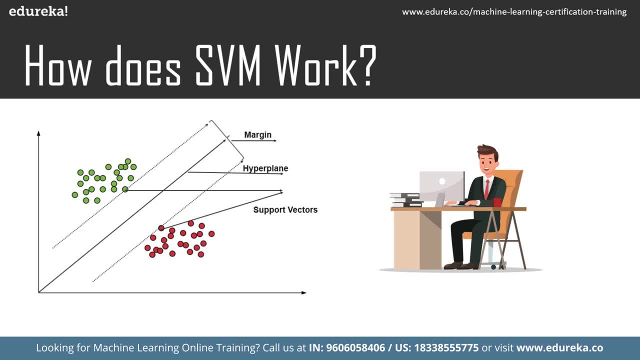 with the maximum segregation from either nearest data points. Now let me tell you how we can deal with inseparable and nonlinear planes as well. So in some cases, hyperplanes cannot be very efficient, and in those cases the support vector machine uses a kernel trick to transform the input into a higher dimensional space. 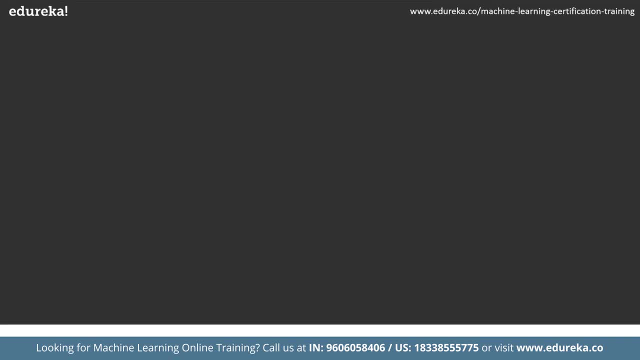 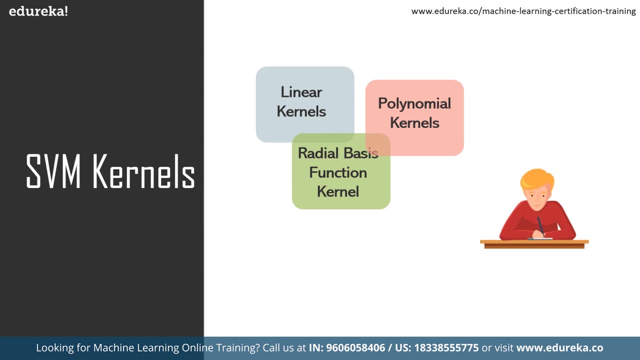 So with this it becomes easier to segregate the points. Now let us talk about the SVM kernels. So an SVM kernel is basically used to add more dimensions to a low dimensional space to make it easier to segregate the data. It converts the inseparable problem to a separable problem. 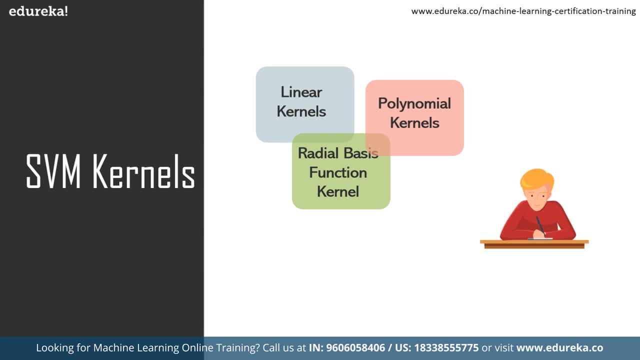 by adding more dimensions using the kernel trick. a support vector machine, or SVM, is always implemented in practice by a kernel. The kernel trick helps to make a more accurate classifier. Let me talk about the different type of kernels that we have in support vector machine. 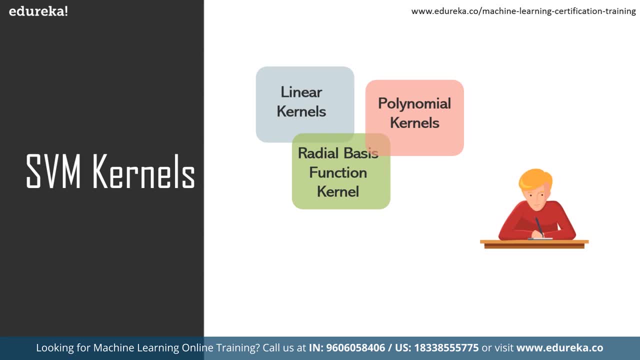 First of all we have linear kernel. a linear kernel can be used as a normal dot product between any two given observations. So the product between the two vectors is the sum of the multiplication of each pair of input values. and then we have the polynomial kernel. 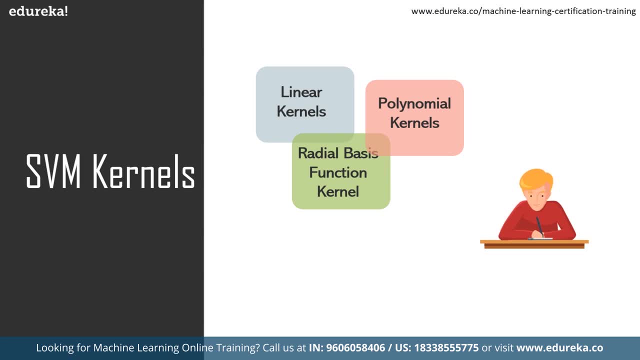 So it is rather generalized form of the linear kernel. It can distinguish curved and nonlinear input space as well. Now, talking about the next kernel that we have, that is a radial basis function kernel. So the radial basis function or RBF kernel is commonly used in SVM classification. 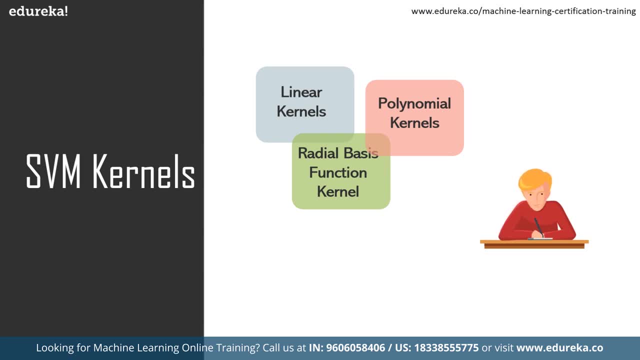 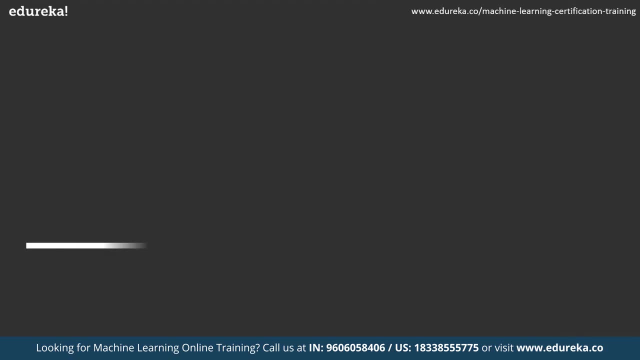 It can map the space in infinite dimensions. That is the advantage that we have with RBF kernel. So these are the kernels that we have in SVM guys. Now I'm going to tell talk about a few support vector machine use cases. So these are a few use cases I have listed down here. 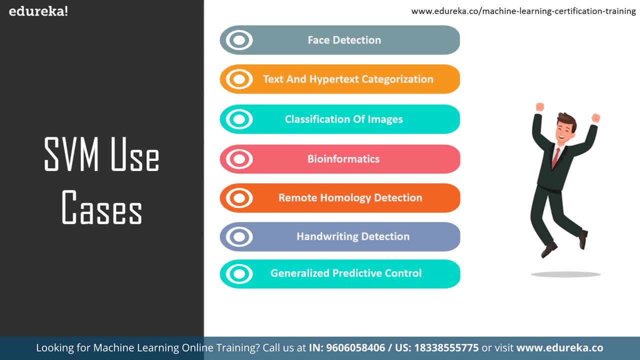 We can use SVM for which is phase detection. can use SVM for phase detection, Then we can use it for text and hypertext categorization. Then we can use it for classification of images. We can use it for bioinformatics, protein fold and remote homology detection. 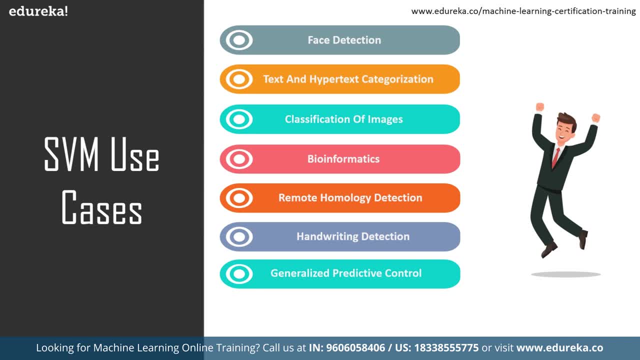 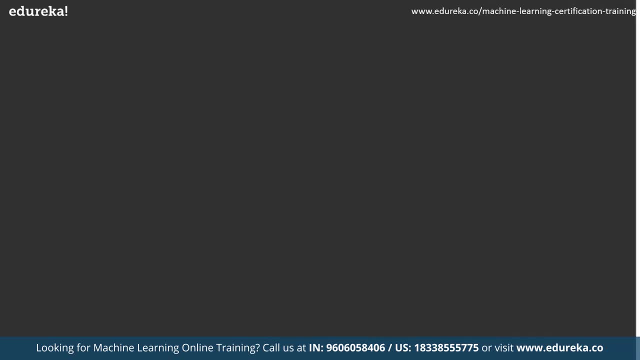 We can use it for handwriting recognition and we can use it for generalized predictive control as well. So these are the use cases that we can use SVM for. now that we are done with the SVM use cases, Let me tell you how we can implement SVM. 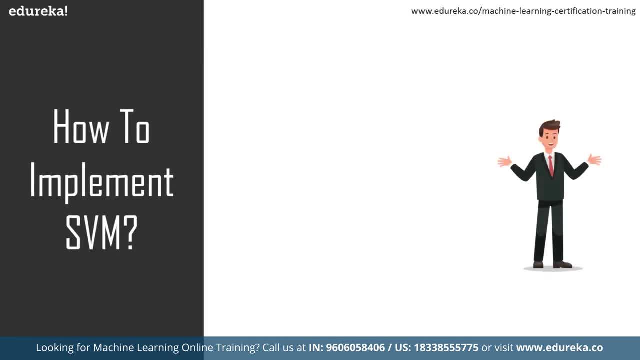 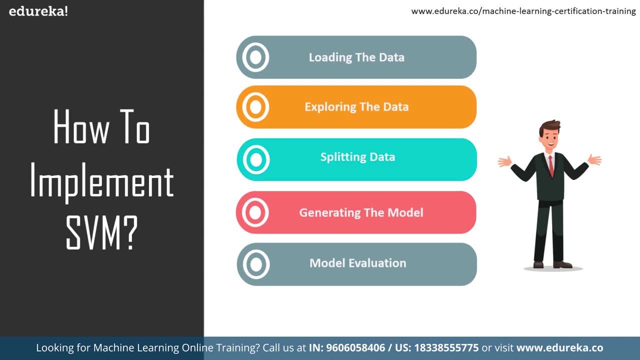 So there are a few steps that we have to follow. to implement support vector machine in machine learning. In any machine learning model, we have to follow specific steps. So first of all, we have to load the data in which we are going to perform. 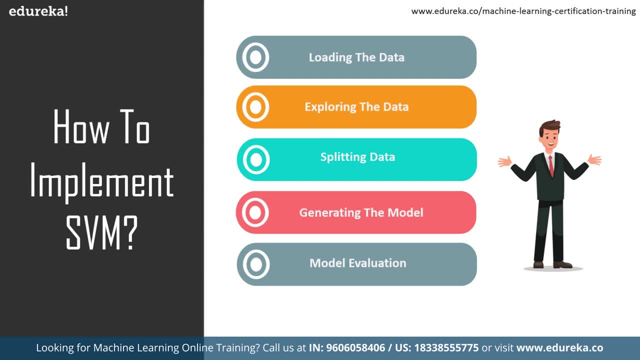 the classification of data. after that We are going to explore the data. We're going to see how many labels, what are the target variables there, and then we're going to split the data into train and test data and then we'll generate the model by implementing the support vector machine. 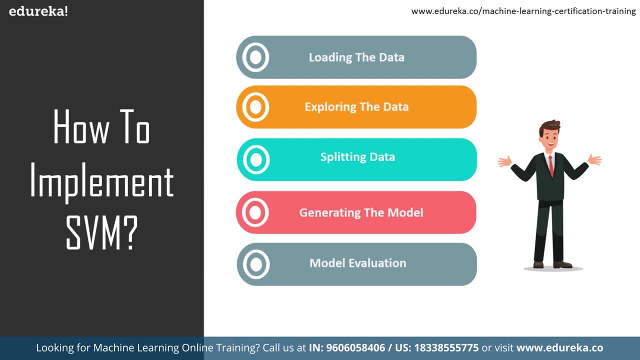 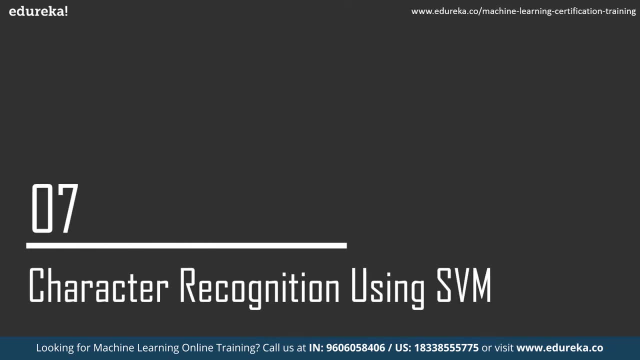 And after that we are going to evaluate the model as well. So I'm going to show you this when we are going to work on the pie charm. after this, I'm going to show you a simple use case, which is a character recognition using support vector machine. 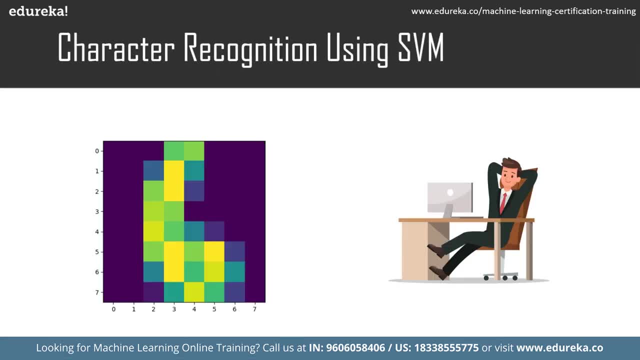 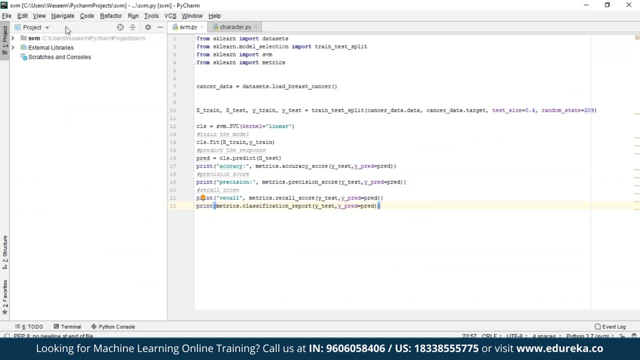 So in this we are going to get image recognition, something like this. So let's take it up to pie charm guys and I'll show you how you can implement support vector machine in Python. So we are in pie charm guys. Let me go to the presentation mode for better visibility. 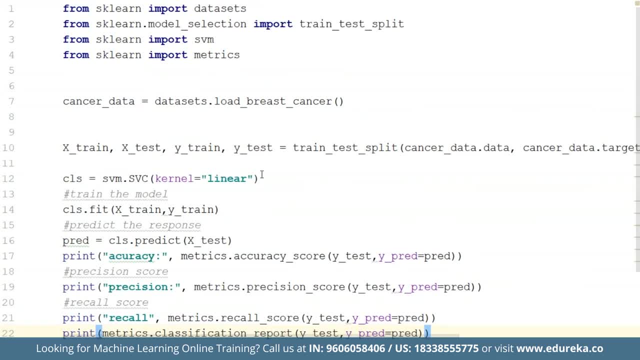 So first of all you have to make sure you have all these libraries installed in your system. that is, psychic learn, SK learn. and then you have to import all these modules like SVM, metrics, train test, split from model selection and data sets to load the data. 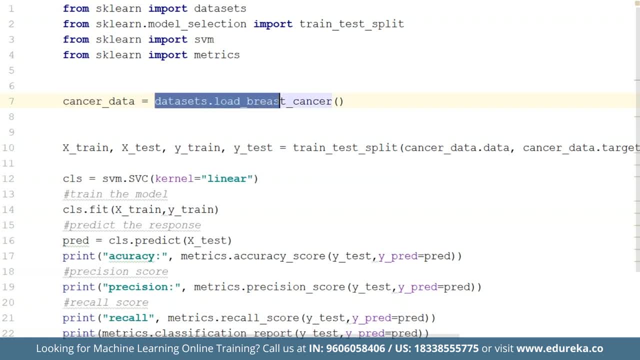 So first of all, we have that cancer data over here in which we are going to load the data set, which is the breast cancer data set. So this is a simple example, or this is the way we can load the data and just write a comment over here. 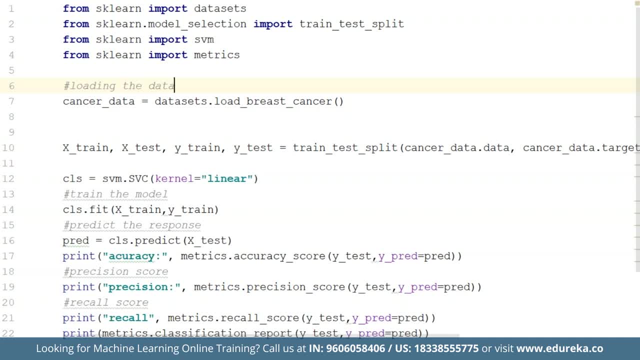 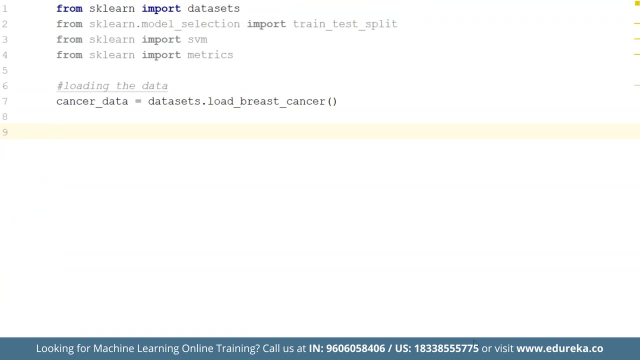 Loading the data. This is where we are going to load the data. after this, We can check for what all are there inside the data, like how many images or what all is there. So I'm just going to remove all this for now And let's see what we have in the data. 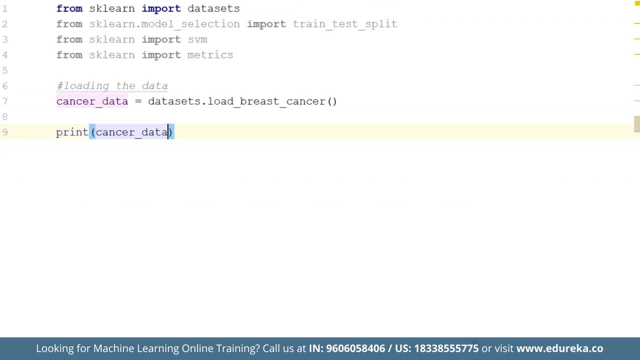 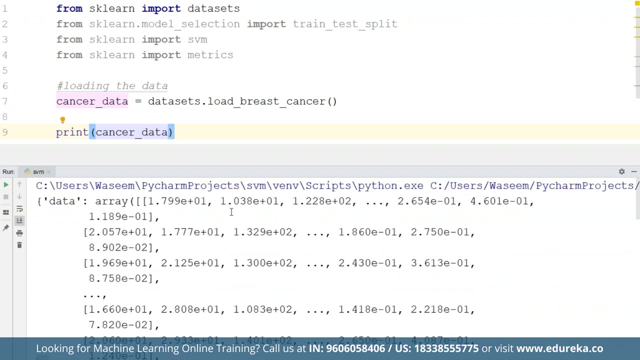 So I'm just going to print cancer data. Let's see what we have. It's going to take a while because it's loading the data set from the internet. You can see these. all points are there inside the data set. So we have data. 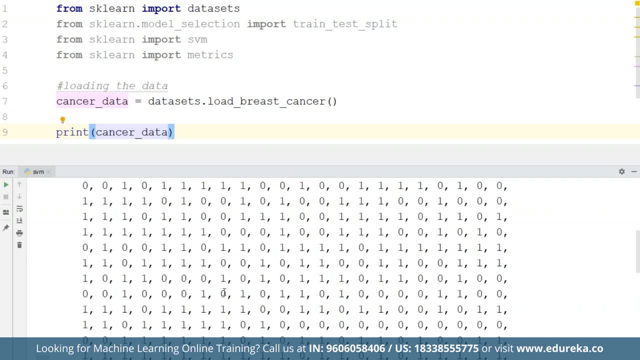 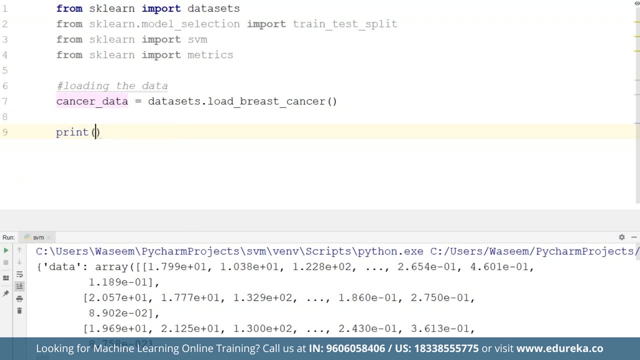 Then we have Target also here, Which is an NP array. This is the data that we have over here. Now I'll just check the shape of the data as well. Let's see the target variable also. So this is our target variable, guys. 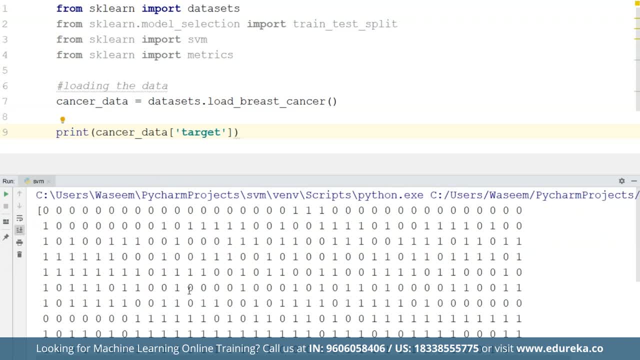 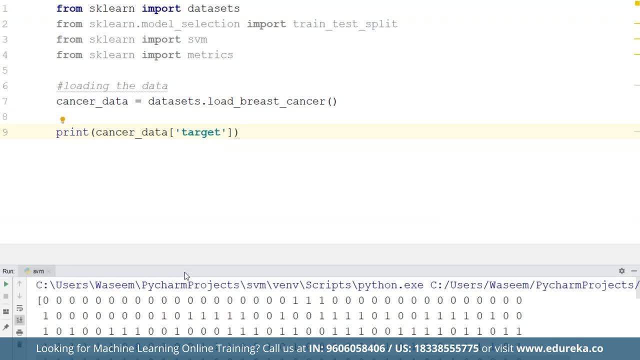 which is in a binomial form, which is 0 and 1.. So we have only two possibilities over here. Now that we are done exploring the data, also, let me show you how you can start splitting the data into test and train sets. 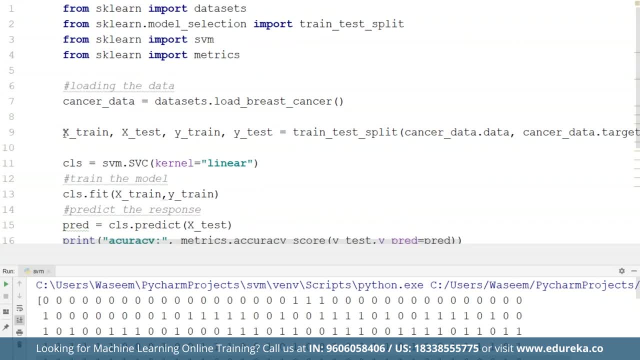 So I'll just remove this again and print the previous code. So this is my training and testing variables. That is X train, X test. We have Y train, Y test and inside this I have used train test split to train my data over here. 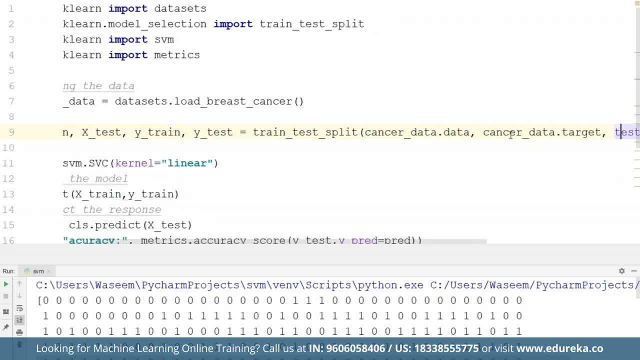 As you can see, I'm using the data as cancer data. Then we have the target variable. We are using the test size at 0.4.. We can use it at 0.3 as well. We'll be using like 30% for the testing. 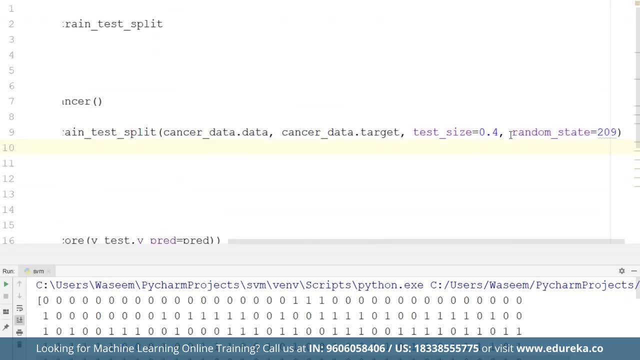 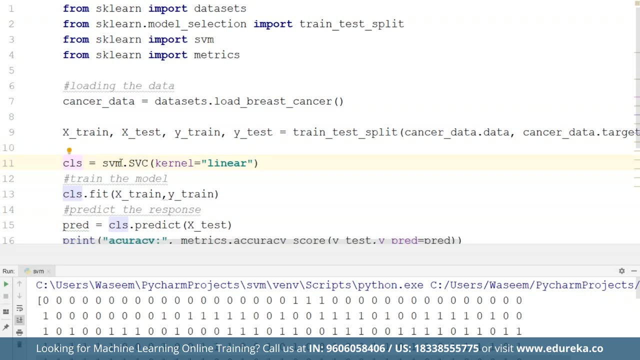 and the other one for training, And we have a random state as 209.. After this, I am going to generate the model- that is my classifier, using the SVM over here and I'm going to use the SVC with the kernel linear. We are using the linear kernel over here. 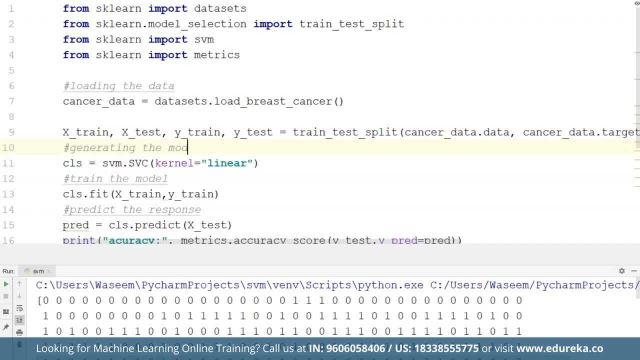 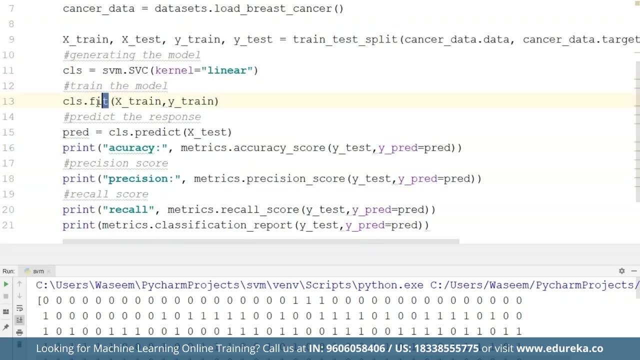 So I'll just write: generating the model. After this, we are going to train the model. for training the model, We are going to use the fit method over here. inside this, We are passing the X train method and Y train method to train the data. 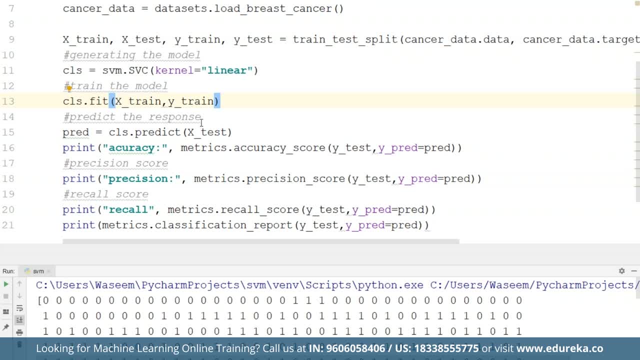 So basically, the fit method is used to train the data. after this We are going to predict the response using the predict method over here. inside this We are going to pass the variable, that is X test. So we have taken the X test separately for this purpose, only to predict the outcome over here. 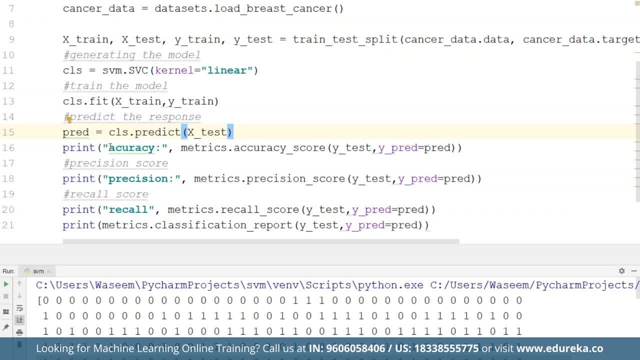 So now that we are done with the training and testing over here, We are going to print the accuracy. I'll just write one more. see over here to make it correct. for this We are using the metrics from the escalian module, which is going to give us the accuracy score in this. 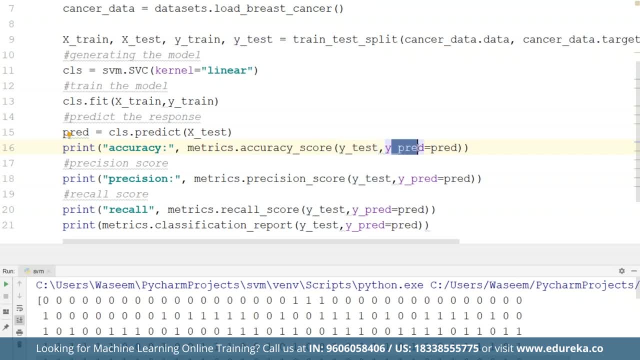 We have Y test and Y prediction, So it's going to give us the accuracy report. after this, We are going to get precision score using the precision score method in Matrix, and then we have recall as well, and to make it easier, I'm also using a classification report. 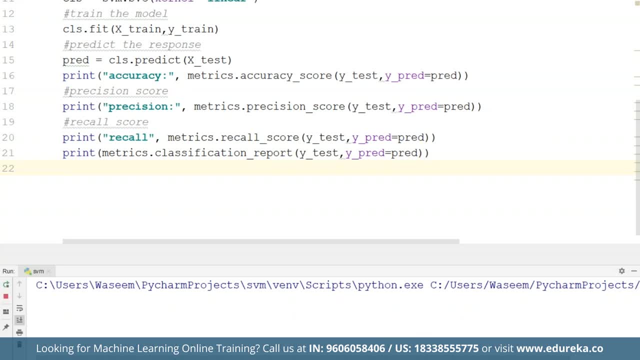 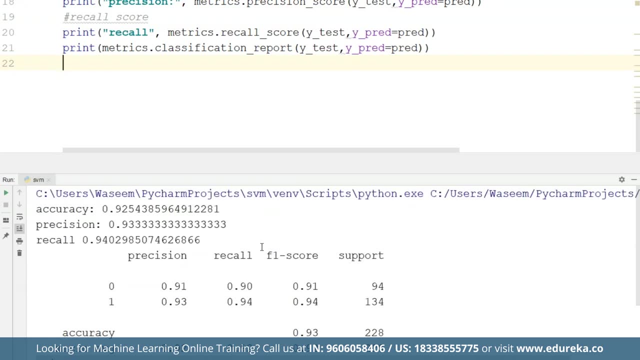 So let's just run this program, guys, and we'll see what happens. We'll get the total report how efficient our model is actually. So, as you can see, we have the accuracy as 0.92, which is close to 92%, and then we have precision of 93%. 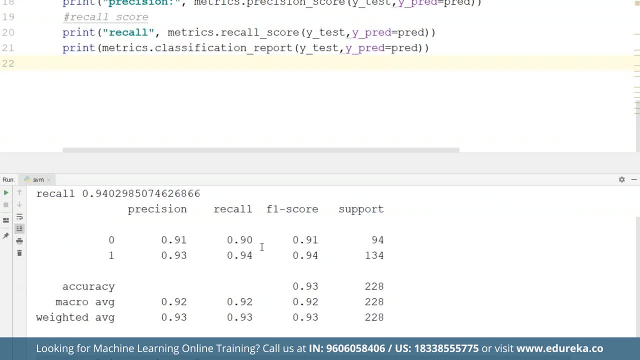 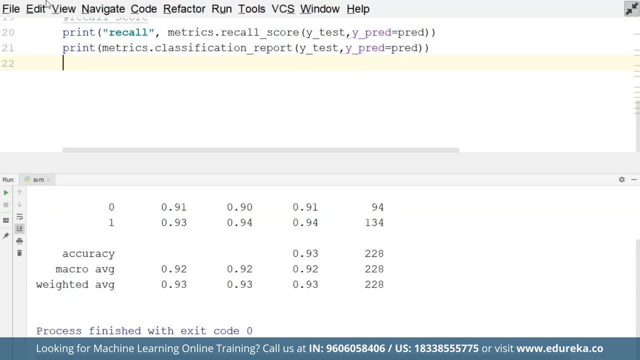 and recall as 94%, and after that we have a classification report. inside this we have also given the accuracy, the FN score and the recall as well. So this is a simple example to implement your support vector machine guys. now moving on, Let me show you one more example before that. 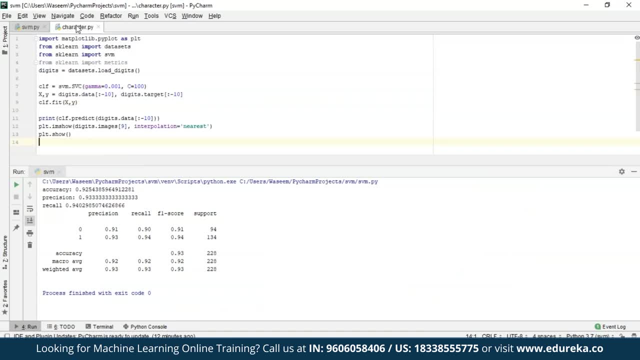 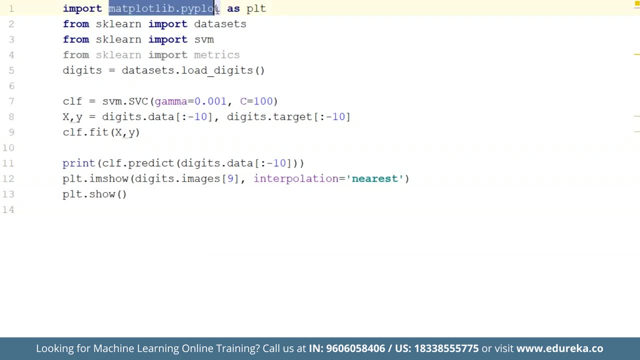 Let me just exit the presentation mode Now, going to show you a use case for character recognition using support vector machine. So for this also we are using one more library, that is matplotlib, To plot the graph or to plot the image as well. So we have data sets which we are going to import from sklearn. 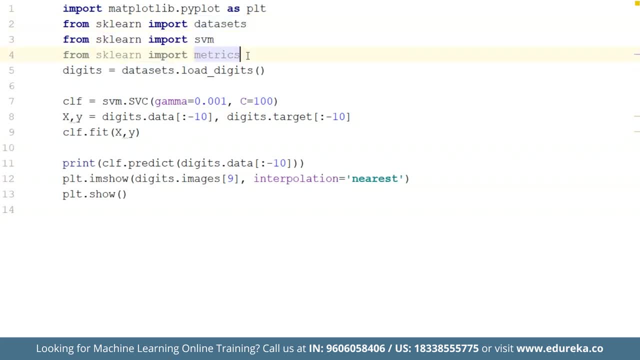 only we have SVM and Matrix, which we are not going to use in this one for accuracy, which I'll tell you later, guys. So first of all we are loading the data sets over here. This is the load digit. So we have a data set with a bunch of digits. 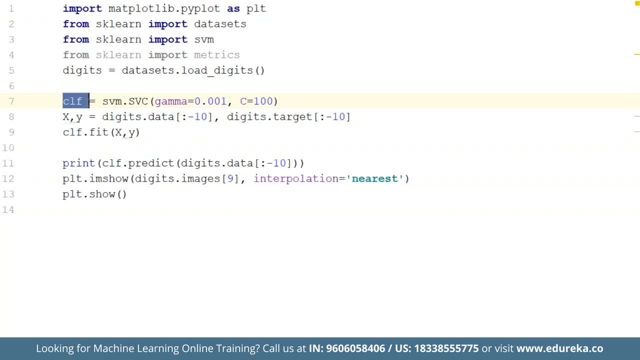 the handwritten digits, and now we are generating the model directly. after this, We have X and Y variables, which is, you know, going to take the test data and the target data as well. So we are taking all the data until minus 10 over here for training. 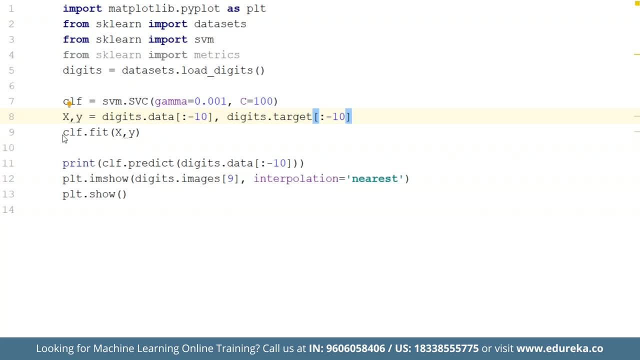 and for target variable, We also taking the same number and after this we are going to fit the model, to train it and we are predicting the models with the digits data. That is over here after this. I'm just going to show a image, or it's rough- 9.. 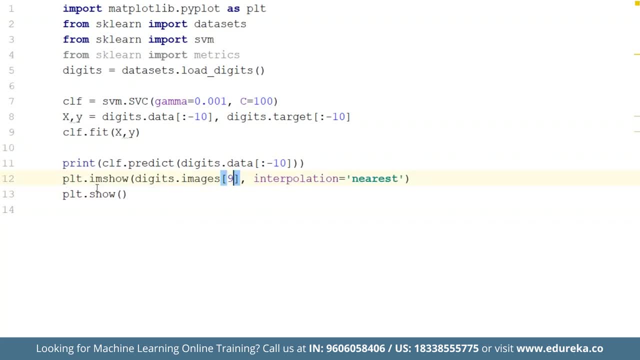 We can use any other number. We have taken interpolation that is nearest and I'm using the. I am show method from the matplotlib And if you are not familiar with matplotlib or how you can plot graphs, you can check out other tutorials in the area on matplotlib to get better insight about this.